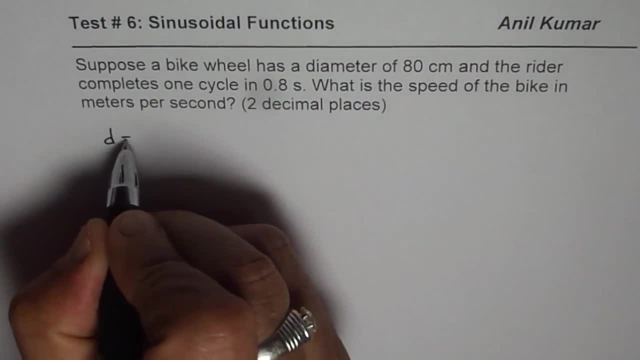 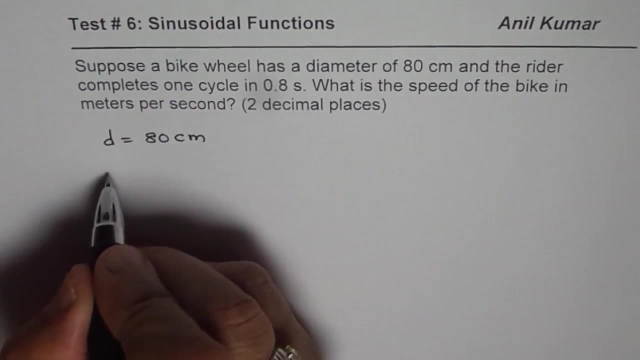 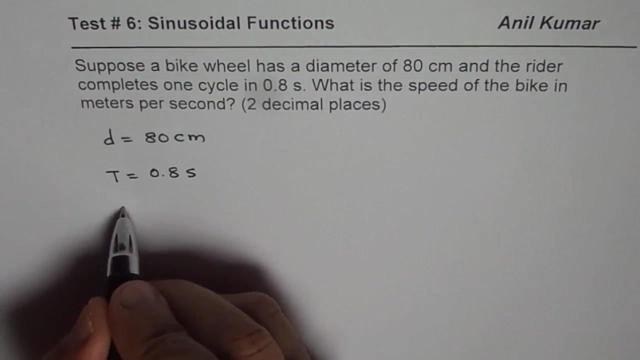 Now, what we are given here is diameter, So diameter is 80 cm, and time taken for one full cycle. So the time period t is 0.8 seconds. What is the speed? So we need speed. You know speed is distance divided by time. So speed is distance divided by time. 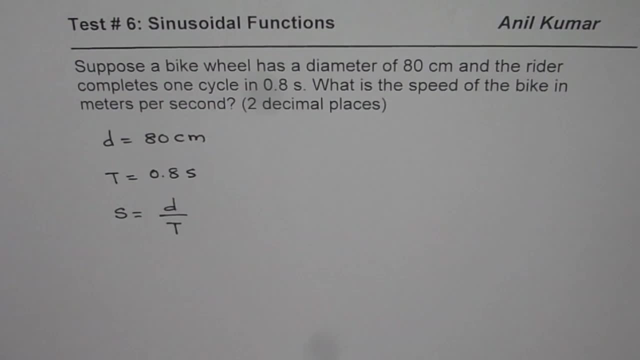 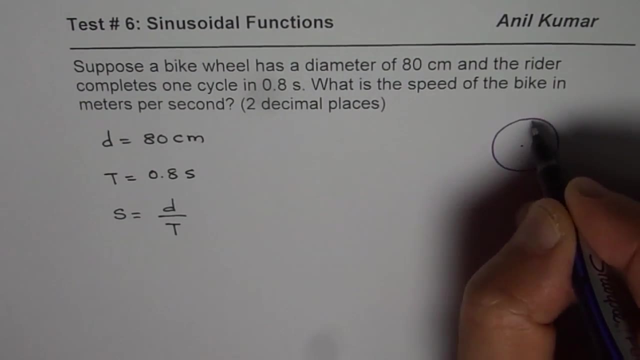 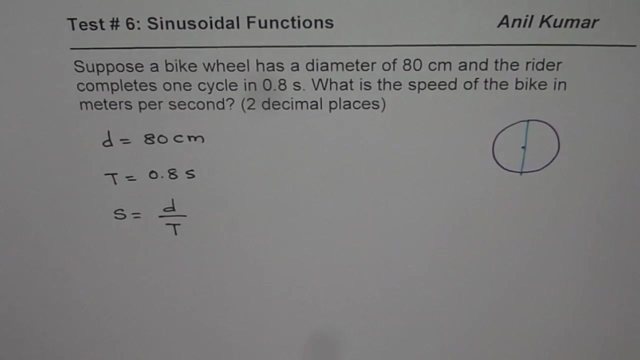 Now, in one cycle, how much distance will be given The bike cover? So this is, let us say, the wheel of the bicycle right, Whose diameter is given to us as 80 cm. Now, how much distance is it going to cover in one cycle? Pi d, right. So distance is the circumference. So you say distance is actually the circumference, which is pi times the diameter, or 2 pi r right, Either way. 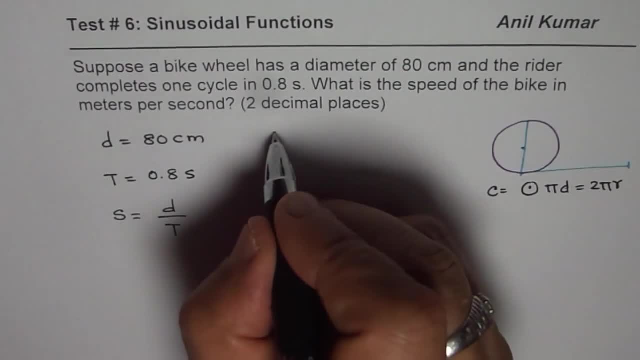 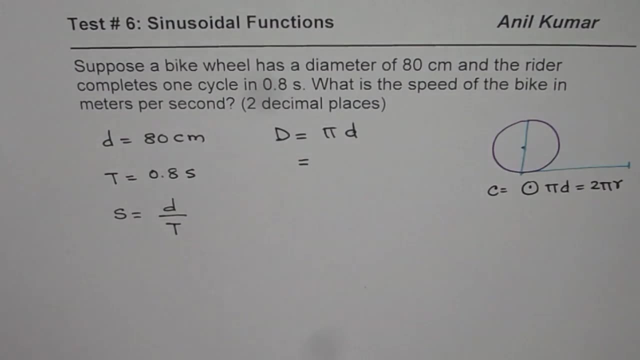 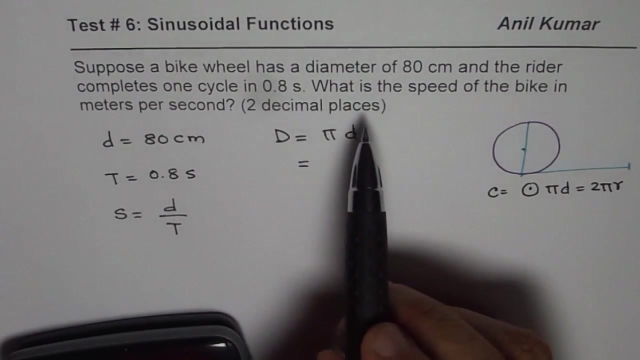 So we can find out the distance. Now what we can do. we can find the distance covered as capital D equals to pi times d, And in our case, pi. we can use the calculator. Since we need two decimal places, we can actually use the value of 3.14 also, right? So in any case, let me hold, get a calculator. And well, one more thing, That is, we need speed in meters per second, So we have to convert centimeters to meters. We just need to read the meter, So we have to write it in the meter. So we have to convert centimeters to meters And we have to write the value of 3.14.. You know, 3.14 is nothing when we translate pi across d in high school math class. So we have to go from 1.7 to 3.14. Same as u over d, over d In general. Now, when can we calculate world speed over 10, because, discovered bei阿İTTFI. 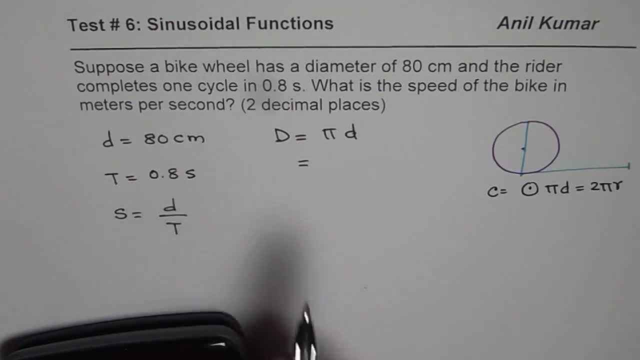 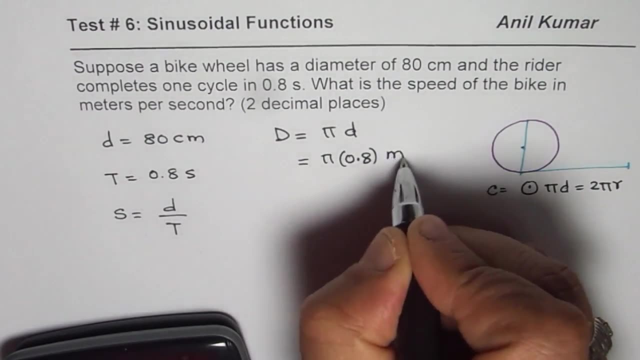 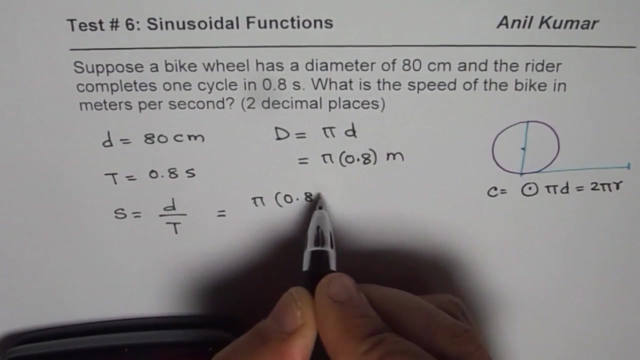 passing tiger continues through delivery. Micro card means the transmission on pickles, or stopehãивa, centimeters to meters, which is 0.8. right, so we get pi times 0.8 meters, as the distance, and therefore speed, can be written as pi times 0.8. 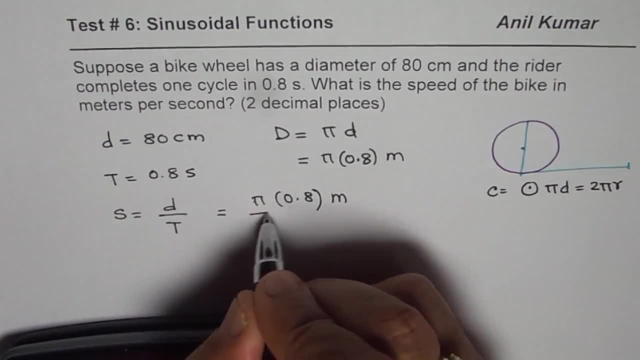 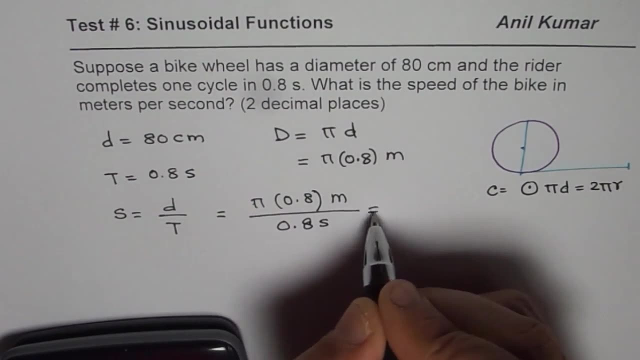 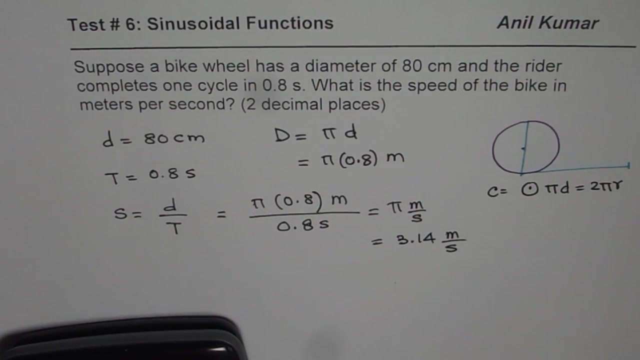 meters divided by time taken for one revolution, which is also 0.8 seconds right, so it is pi meters per second. to two decimal places, it is 3.14 meters per second right. so that is our answer for the given question. thank you.